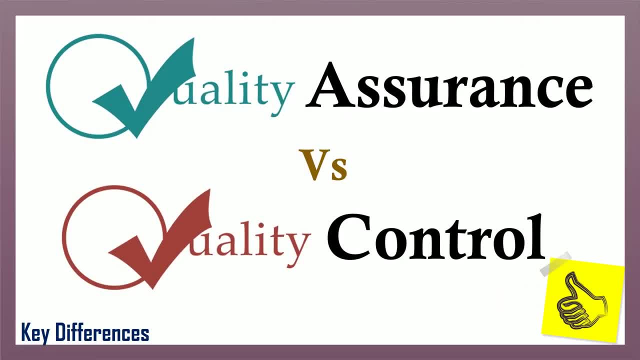 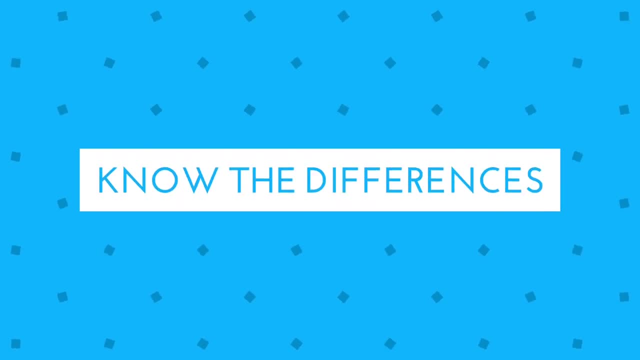 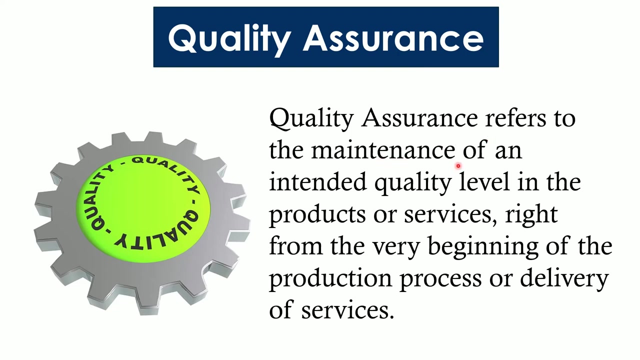 Hey guys, I am Surbhi and once again welcome to my channel. Key Differences. In this video we are going to talk about the differences between Quality Assurance and Quality Control. So, friends, let's get started. Quality Assurance: Quality assurance refers to the maintenance of an intended quality level in the products and services right from the very beginning of the production process or delivery of services. It prevents faults, losses, waste and defects in the manufactured goods to provide sufficient confidence that the product will meet the requisite quality. Basically, there are two principles of quality assurance. 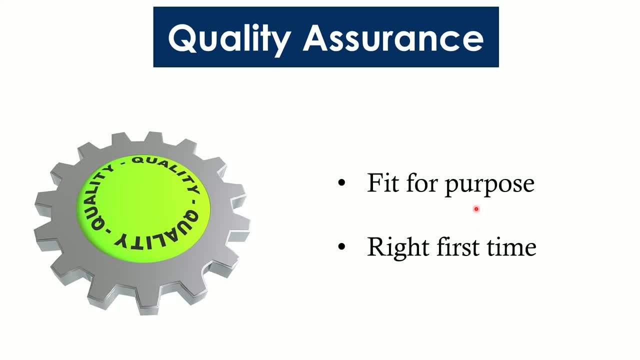 Quality Assurance Fit for purpose and right first time. Fit for purpose means the product should fit the desired purpose, That is, the product should serve the purpose for which it has been developed. On the other hand, right first time, also called as zero defect approach, It means that the quality must be maintained right from the very beginning of the production process, So that it is free from any defects. 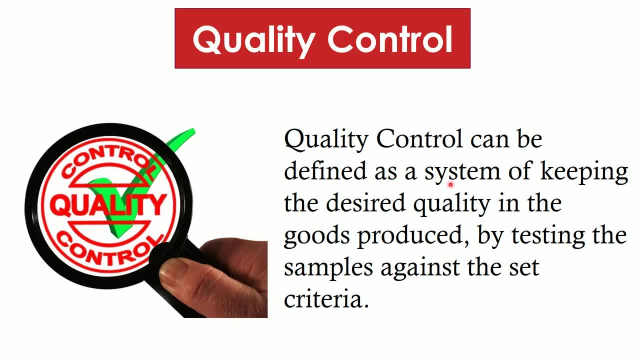 Quality Control. Quality Control refers to a system of maintaining the desired quality in the goods produced by testing the samples of the goods produced against the set criteria. It aims at ensuring that the product and the production process are not just consistent, but they also adheres to the customer requirements. This is possible by providing training to the personnel, setting benchmark for the product quality and testing the products through various techniques to check if they are in line with the set standards. 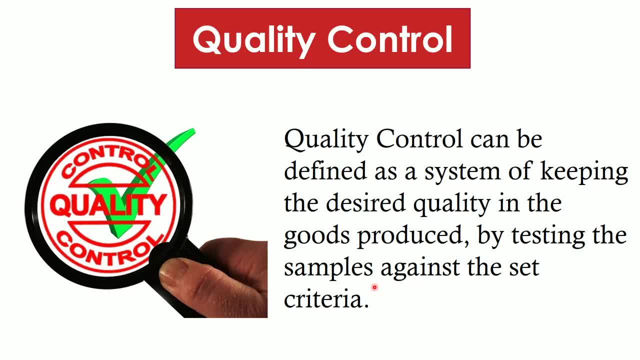 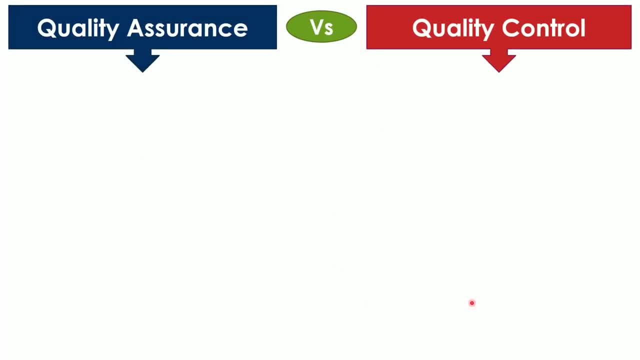 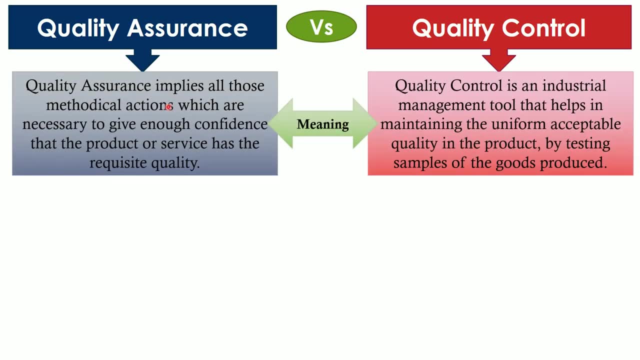 C���: Quality Confidence. Quality assurance refers to a systematic technique of maintaining the desired level of quality services that better meet the demand for the quality of the goods produced in the game Aquí. Quality Control, Quality, Wellness and Qualityammediness management tool that aims at maintaining a uniform, acceptable level of quality in the 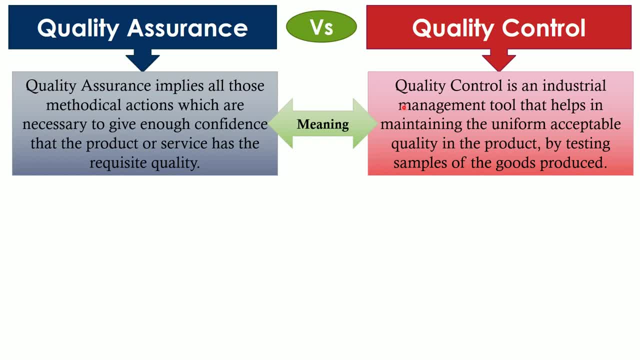 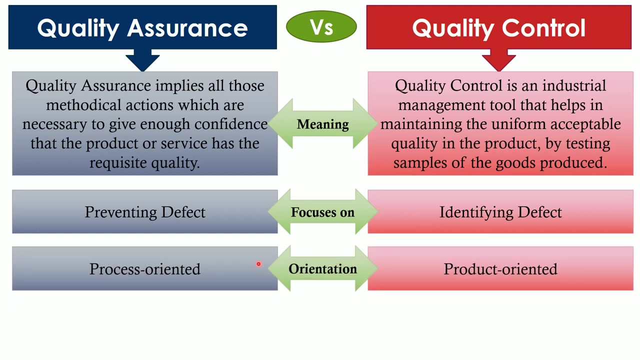 products by testing samples of the goods produced against the set criteria. Focus: While quality assurance focuses on preventing defects from arising, quality control focuses on identifying defects in the products by verifying the samples against the set benchmarks. Orientation: While quality assurance is a process-oriented technique, quality control is a product-oriented technique. 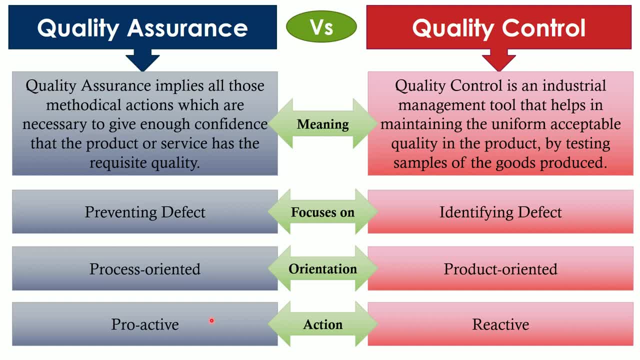 Quality assurance is a proactive method, as it prevents defects from arising by maintaining the quality right from the very beginning. As against, quality control is a reactive method, as it checks the quality after the products are manufactured to identify if the products are not being manufactured. 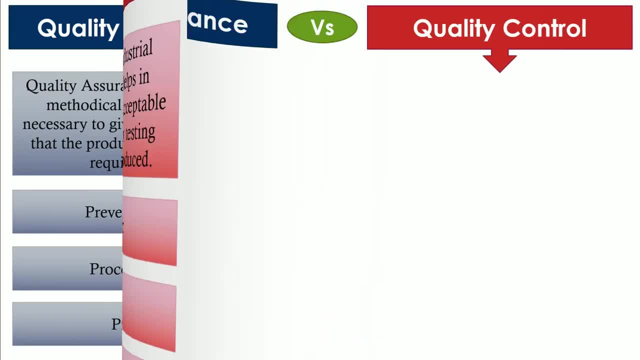 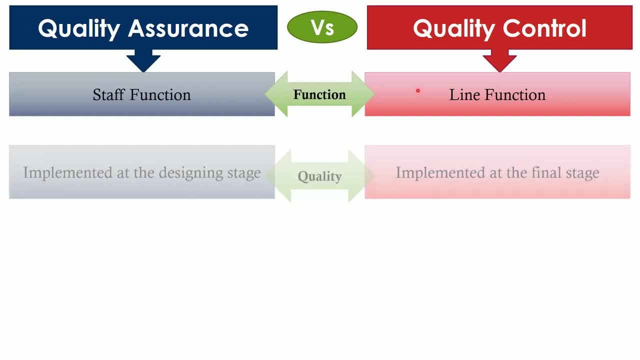 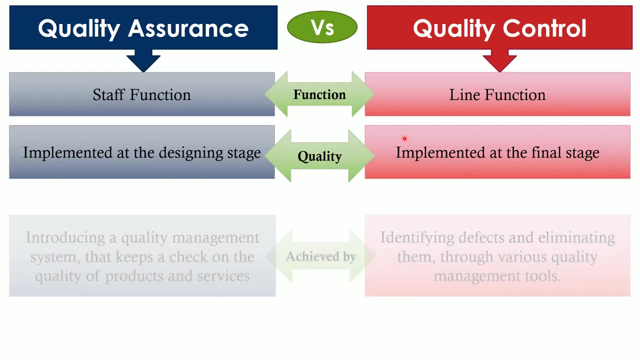 Next, while quality assurance is a staff function, quality control is a line function. In quality assurance, quality is implemented at the designing stage, whereas in quality control, quality is implemented at the final stage, ie when the outcome is produced. Quality assurance can be achieved by introducing an effective and effective quality control. 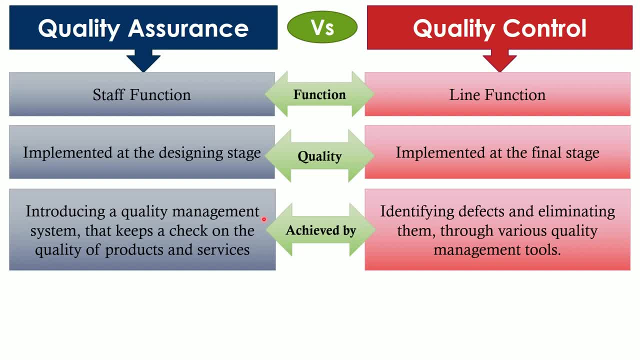 regularly understanding when a product is manufactured to ensure a fruitful and significant overall similarity of material coming from any form, time and quality. The objective quality management system that keeps a check on the quality of products and services at every stage of production As against quality control, can be achieved. 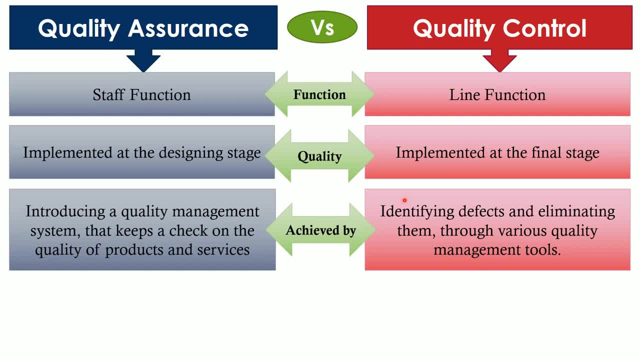 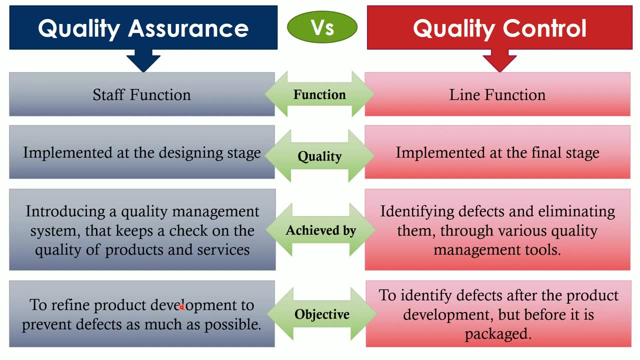 by identifying defects in the products and eliminating them by using various quality management tools. Objective 1. Quality Assurance. The primary objective of quality assurance is to refine the product development to prevent defects as much as possible. Objective 2. Quality Assurance. Objective 3. Quality Assurance. 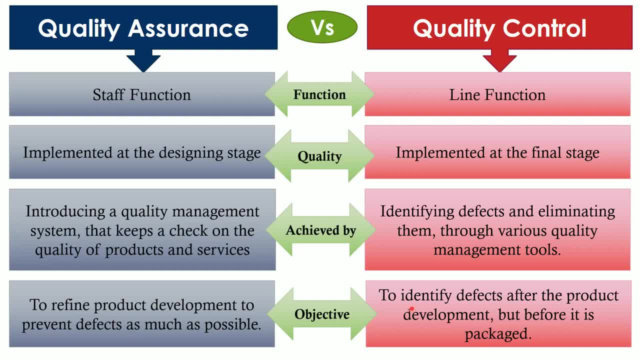 Objective 4. Quality Assurance Objective 5. Quality Assurance Objective 6. Quality Assurance Objective 7. Quality Assurance. The primary objective of quality control is to identify defects after the product is developed through testing, but before it is packaged. So, guys, this brings me to the end of this lesson. 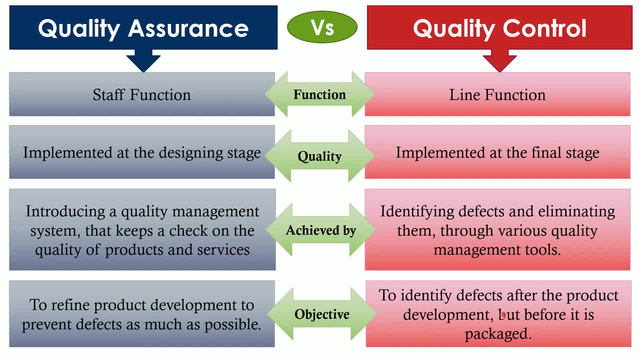 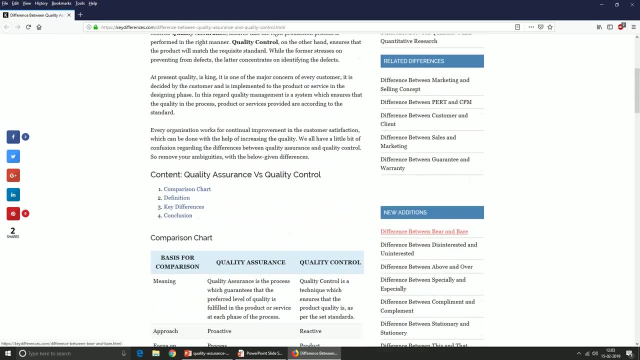 I hope you find the lesson very useful and all your doubts regarding the difference between quality assurance and quality control are clear now. However, if you want to study the topic further in detail, you can visit our official website, that is keydifferencescom. Here you can find a detailed comparison of